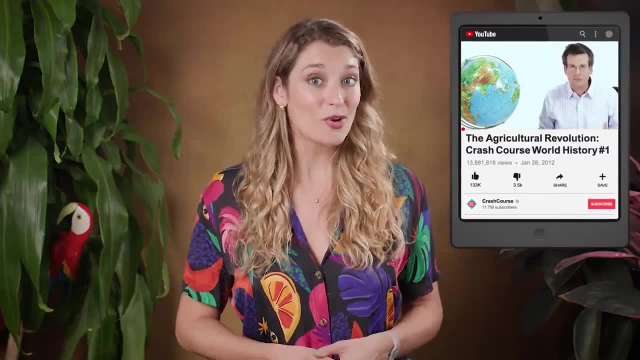 One of the biggest changes in our history and the one pretty familiar to us here on Crash Course, happened about 15,000 years ago, when some humans began to shift from hunting and gathering food to cultivating crops. And that's because language is a very important part of our culture And it's a 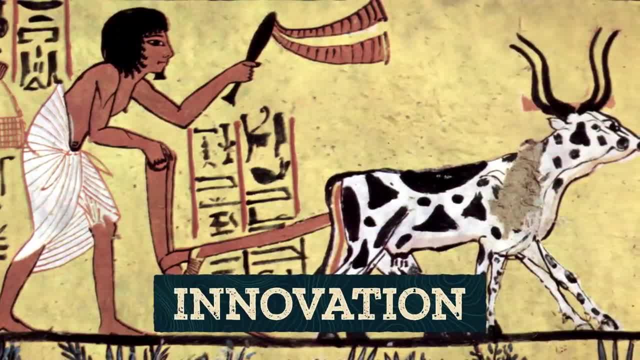 very important part of our culture, And that's because language is a very important part of our culture. Agriculture was a major innovation or cultural change that came from within different cultural groups. In fact, several groups independently invented agriculture and with it, a whole new 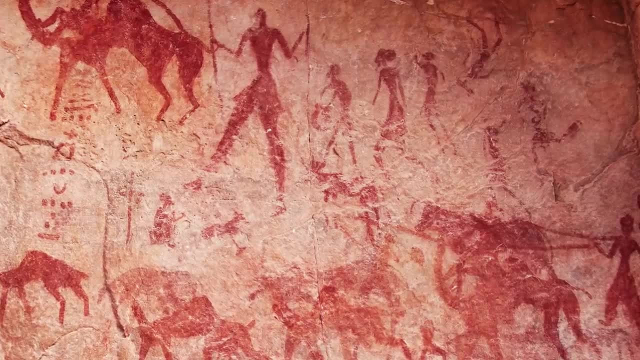 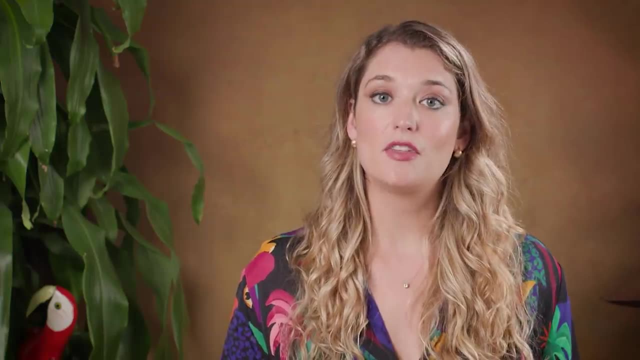 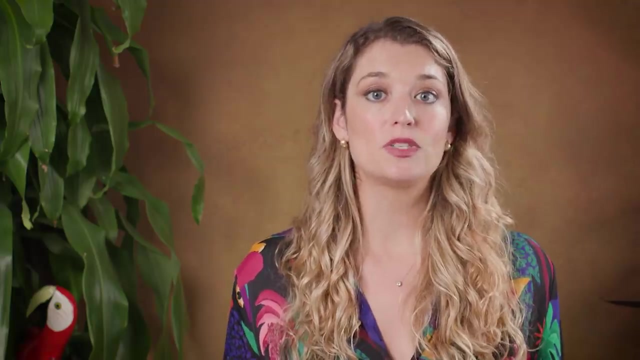 way of life with new social systems. But there have been many more innovations before, after and during the agricultural revolution, like cave art or steel beam architecture. Eventually, populations increased and there were territorial disputes between hunter-gatherers and agricultural communities, Which might not seem important for language, but as different groups. disputed and negotiated territory. they had to deal with each other And that's why we have to interact, and this was one way cultural traits like language were shared. Today we can map out particular cultural traits to see where they're used and maybe get a sense. 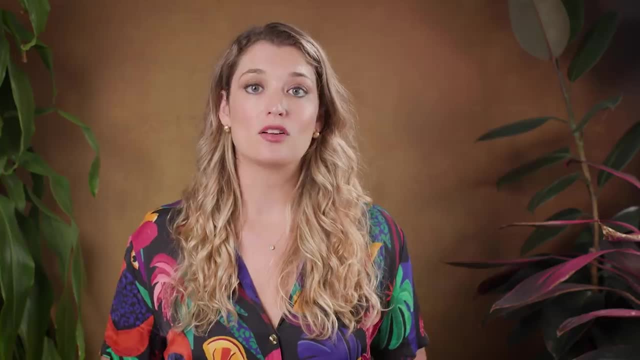 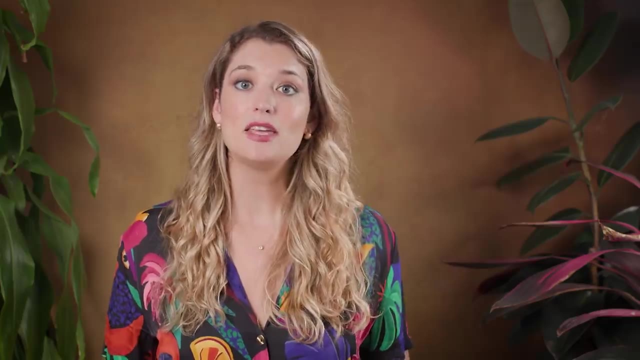 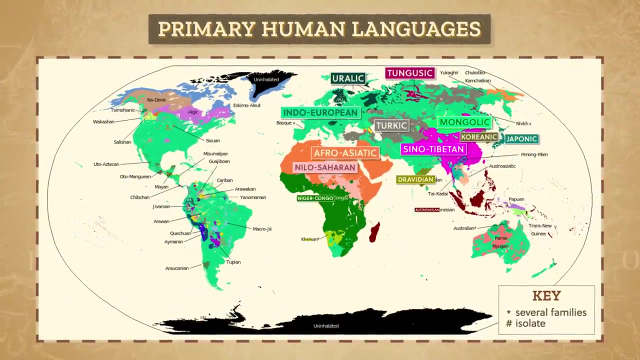 of their journey over time. We might have to dig through historical records, anthropological studies, libraries and museums too, But visualizing cultural traits spatially like this can maybe even uncover the cultural hearth or origin of a trait, Which is what happened with language. Language as a whole can be broken into major language. 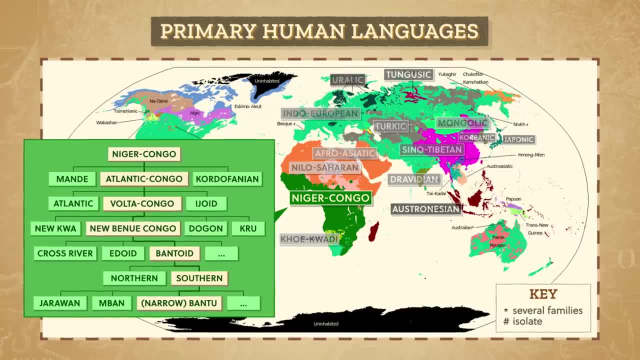 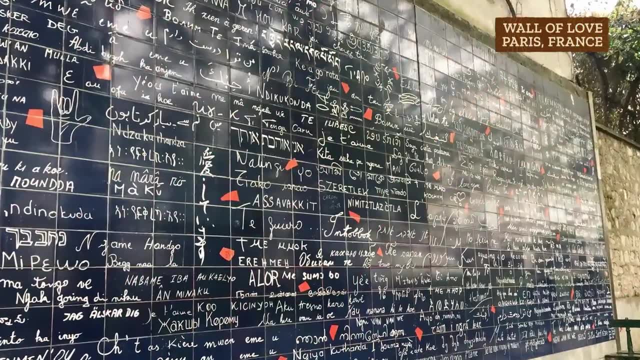 families, from which all of the specific languages we speak branch out like a tree, And each family is a group of languages with a common origin or linguistic hearth. There are roughly 7,000 spoken and signed languages actively used around the world today. 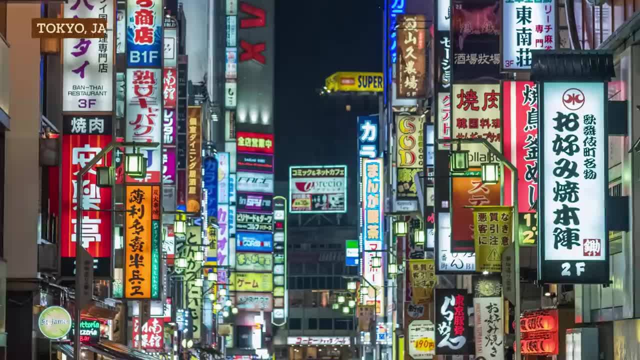 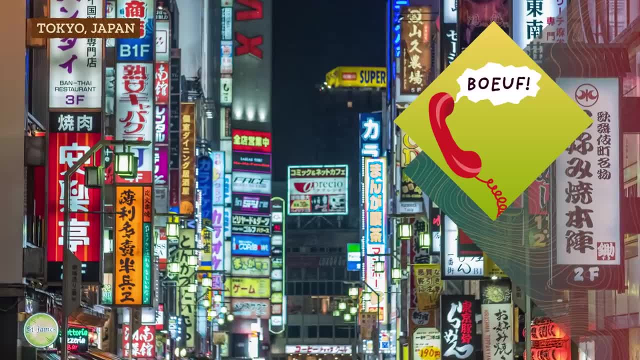 And it's difficult to know how many- have stopped being used over the centuries. Language is key to communicating, and languages, phrases or even individual words have been borrowed and mangled, like we're playing an uncountable number of games of telephone all at once. In geography, we call this diffusion, which is a way to understand how. 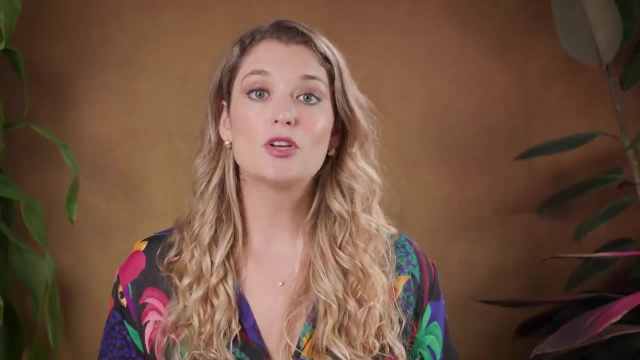 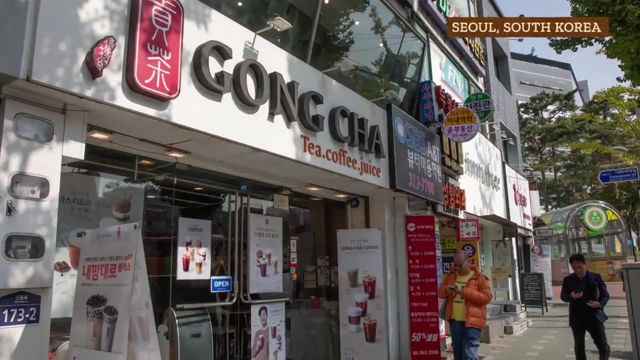 ideas and things move around the world. So with T that original word branches from the Sino-Tibetan family through the Sinastic language group. From there Mandarin branched out. Not all Sino-Tibetan languages would have had the word cha at first. 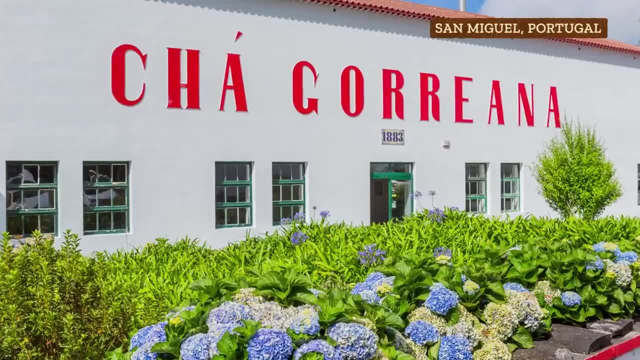 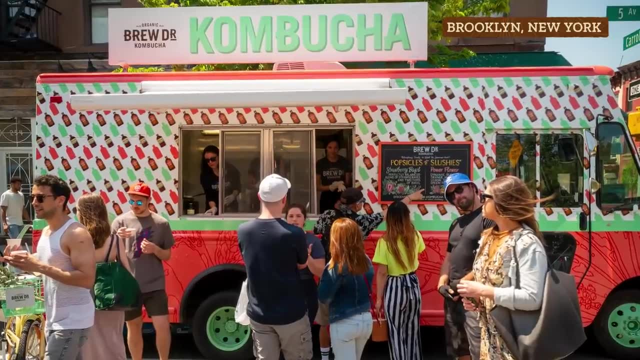 This is one of the largest language families in the world, But those who spoke Mandarin and Cantonese did have cha, and when people speaking other languages learned it, they modified it and worked it into their own language, And on and on diffusing through other languages. 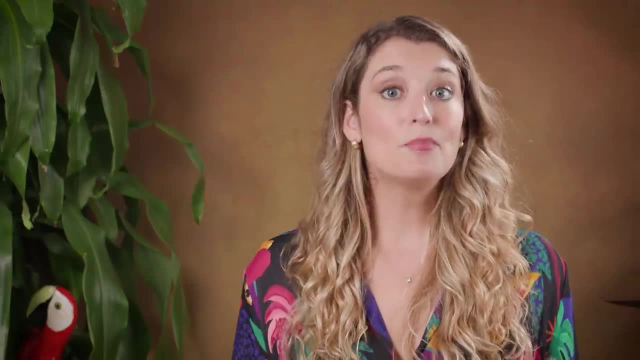 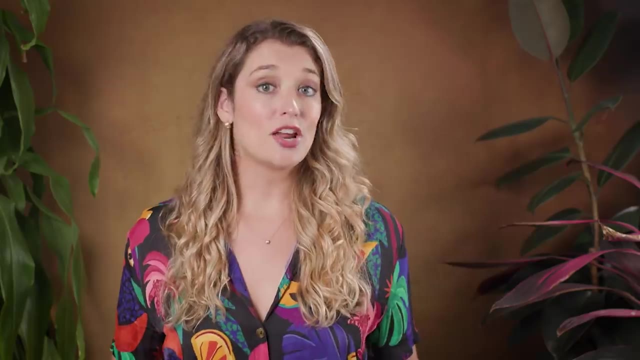 Which would be really cool to visualize Different cultural traits imprint on the landscape in particular ways that we can see And can map, Which is part of how we can locate different cultural hearths. In general, languages can be hard to map Because people can speak more than one language. 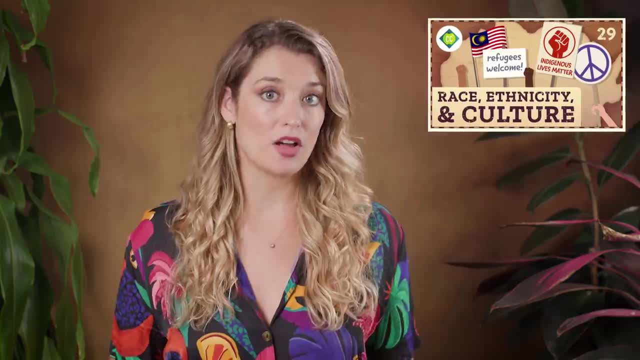 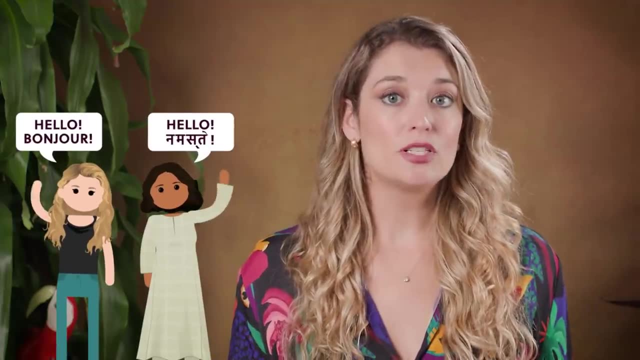 And, as we mentioned last time, sometimes one language has more power than others and it isn't always easy to know the full extent of where a language is used. Like Zora and I, are pretty lucky because by knowing two languages, we can communicate in a large number of places around the world. 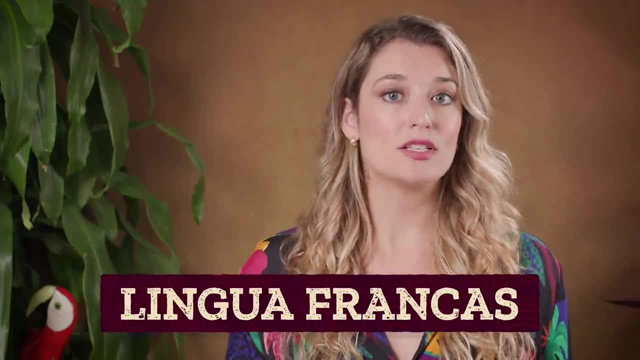 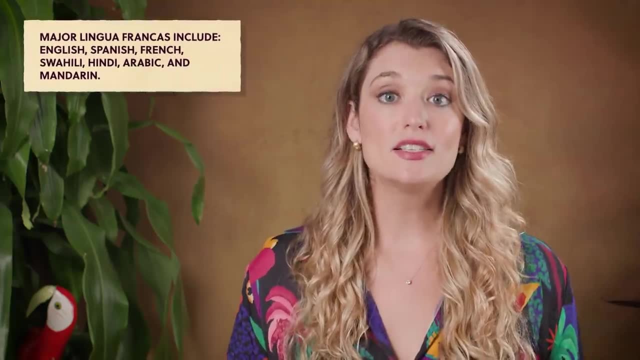 English, French and Hindi are all lingua francas, languages that were adopted in an area to make communication easier between people who don't originally speak the same language, Like for trade. In fact, there are dozens of lingua francas around the world And in a place like Sub-Saharan Africa. 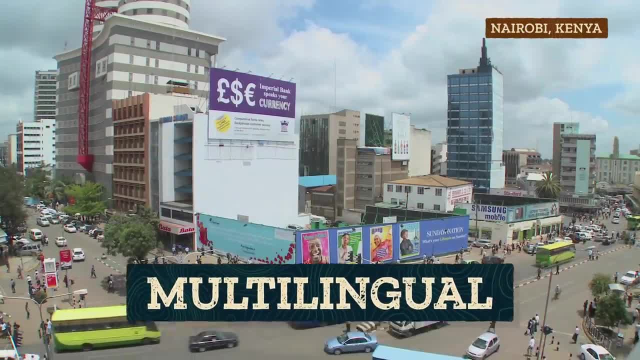 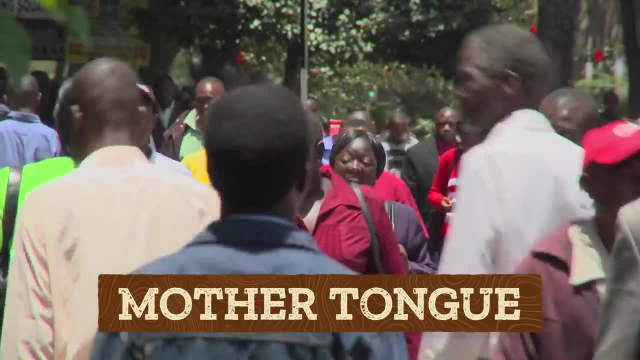 many people are also multilingual, meaning they speak more than one language. People of different ethnicities may share an official language, but also have a language they speak at home or mother tongue and even a local language. And we haven't even gotten into dialects or accents. 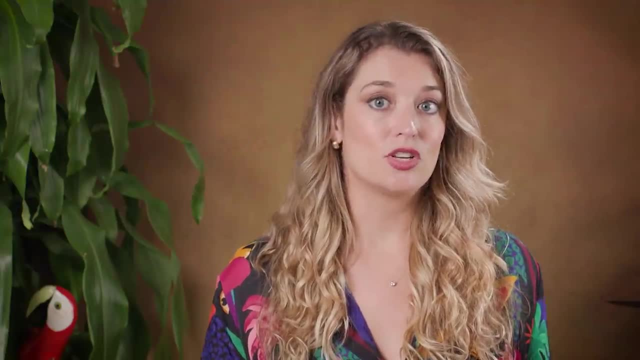 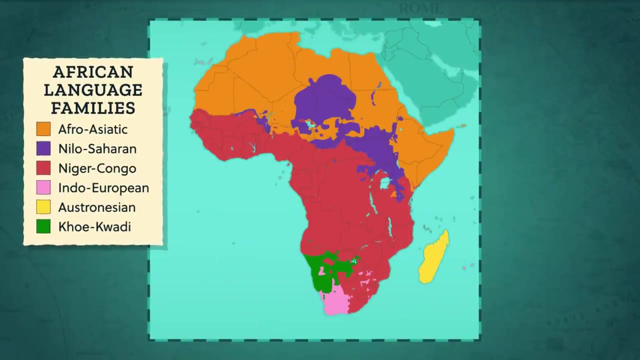 So the location of ethnic groups or people who share the same heritage is one reasonable way to approximate who uses what language where A large continent like Africa is home to about six language families that grew and diffused out of the four to five major linguistic hearths of Africa. 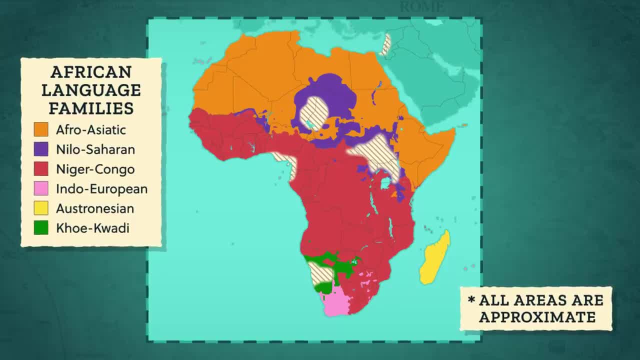 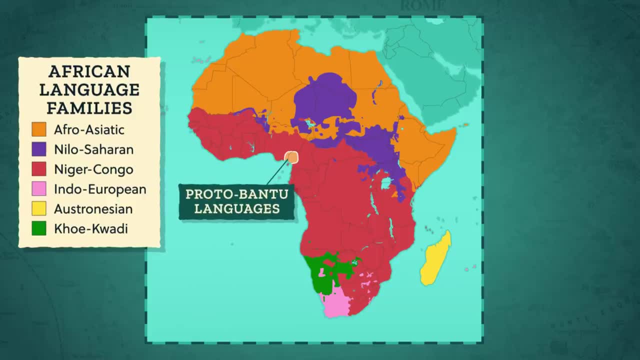 There are at least thirteen sub-families and then hundreds of local languages that developed from there. Specifically, we know the region around what we now call Nigeria and Cameroon is home to the beginnings of what is known as Proto-Bantu languages, which are languages that were spoken about 5,000 years ago in this region of Africa. 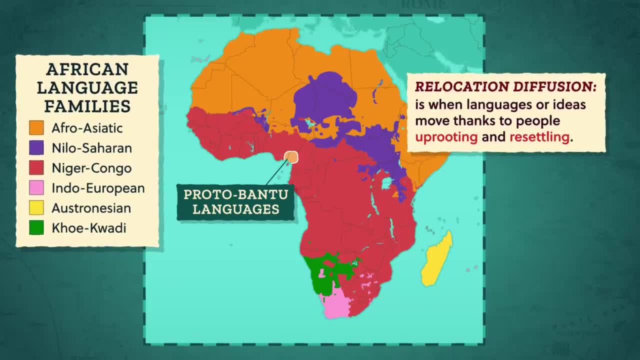 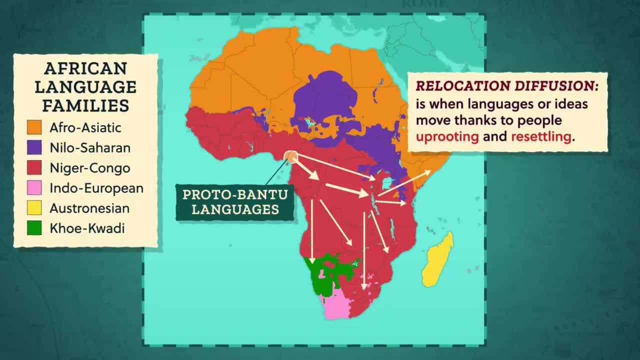 Language is often shared through a type of relocation-diffusion, which is when languages or ideas move thanks to people uprooting and resettling. As the people here moved, they took their language and knowledge of agriculture with them and encountered other groups speaking non-Bantu languages. They'd modify their own language to incorporate some of those words, And geographers and linguists used those words and other elements to reconstruct how language has changed and which languages influenced those changes, Like a few Bantu-based languages in southwest Africa have click consonants. 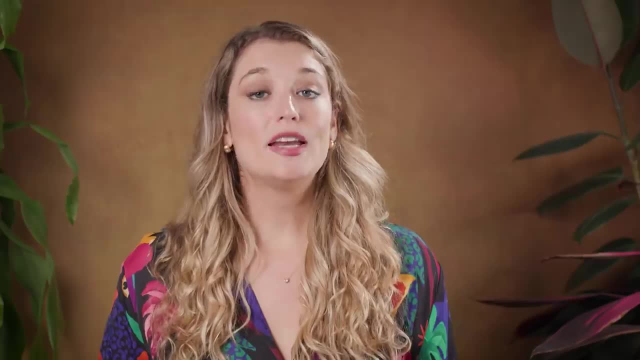 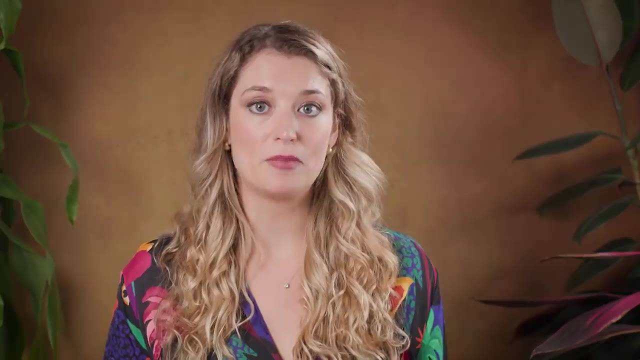 which we think mostly come from the influence of Khoisan languages. For any similar languages we can look at where they're spoken and their structure to put together the connections and imagine the places both groups of people were in to influence each other, Both for ancient and more modern populations. Though we can also lose languages through diffusion. As people move, their languages change or are replaced with new languages, and some languages end up going dormant or no longer having proficient users. Often, as people move or are occupied by other cultures, there's pressure to assimilate. 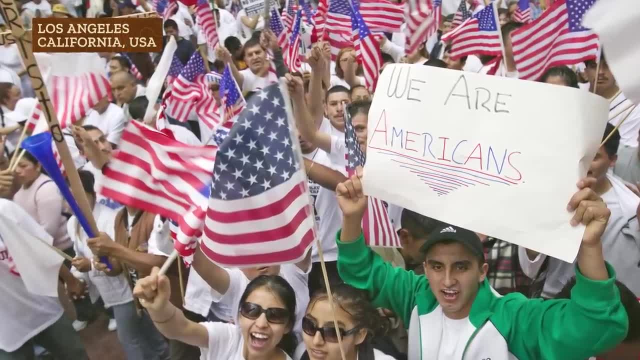 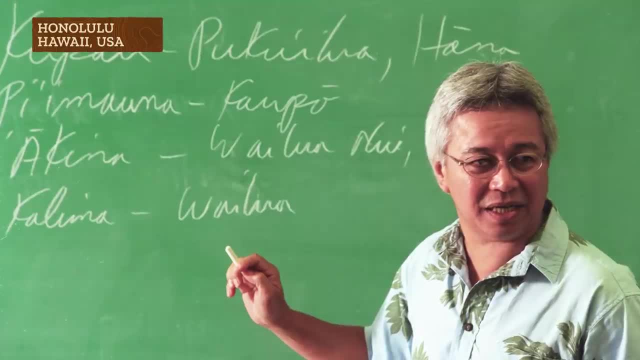 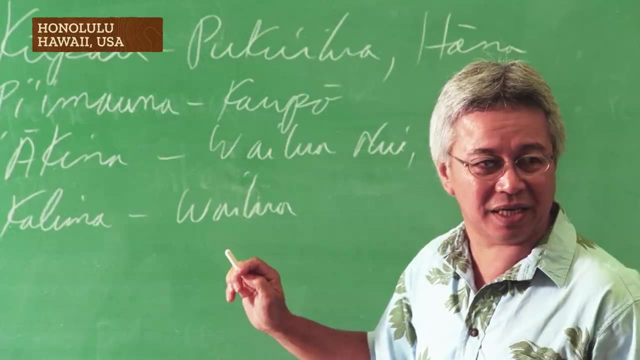 or give up their cultural traits in favor of another set of cultural traits. There can especially be pressure on immigrants or indigenous peoples to change their languages And, after decades of forced assimilation across North America and South America and Australia and the Pacific Islands, there are now efforts to revitalize dormant indigenous languages. 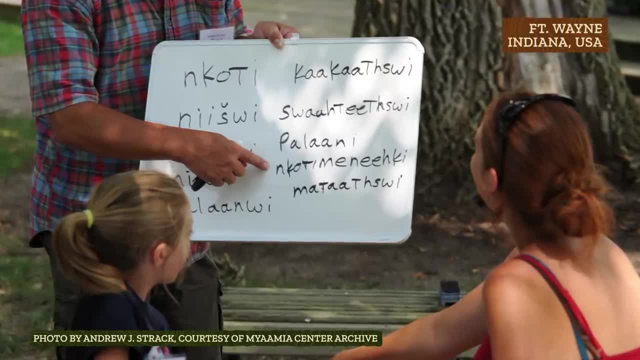 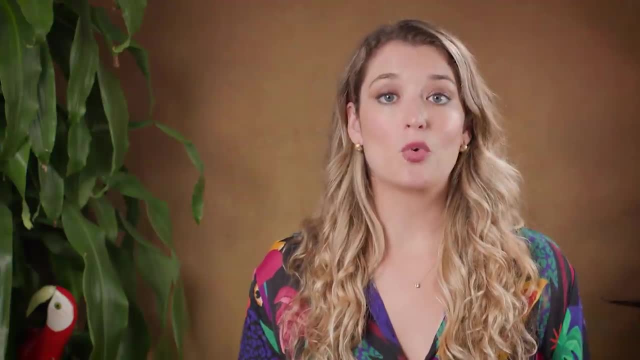 Both the Hawaiian and the Mia-Mia or Miami nations have programs to train preschoolers and other education programs that immerse students in the Hawaiian or Mia-Mia language. Other nations around the world have put in similar efforts, And online, the Endangered Languages Project creates a space for people around the world. 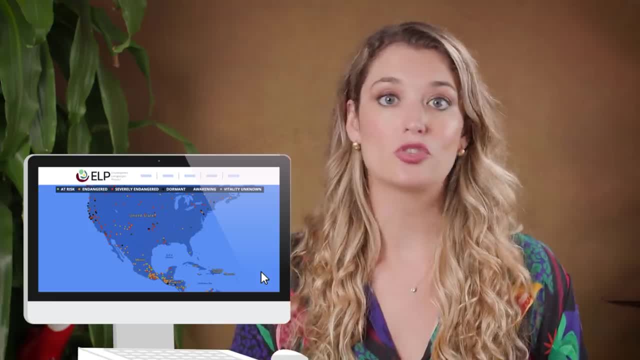 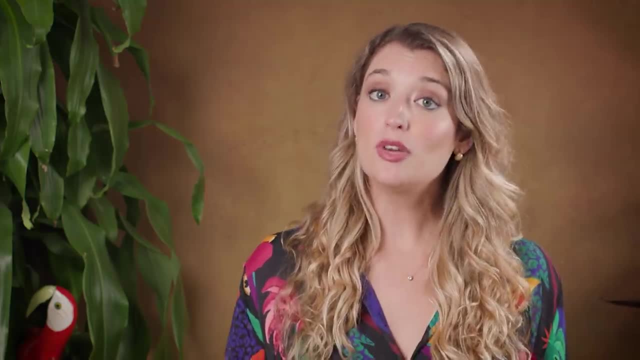 to come together to preserve and revive languages and other cultural traits at risk of going dormant. Cultural identity is deeply personal and living out that identity and living out all of the traits of that culture, including language, can help people feel an important connection to their history and community. At other times. diffusion and the daily mixing of cultures can cause cultural traits to evolve without one language going dormant, Like one of the earliest recorded languages considered a lingua franca was born out of utility. Trade on the Mediterranean was huge in the 1200s. 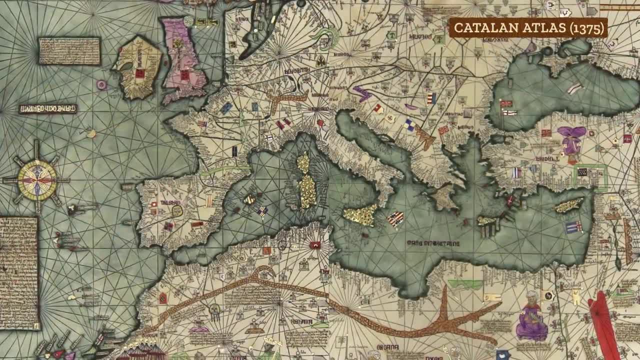 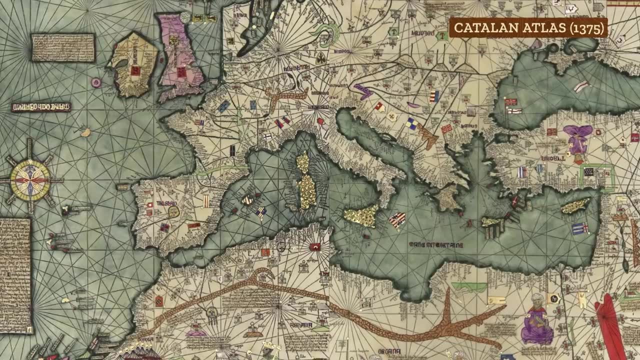 But as people tried to trade their goods, communication got in their way. People struggled to identify languages they knew in common, and when they found words, everyone knew they would use that. Eventually, this created a pidgin or a simplified language, and small. 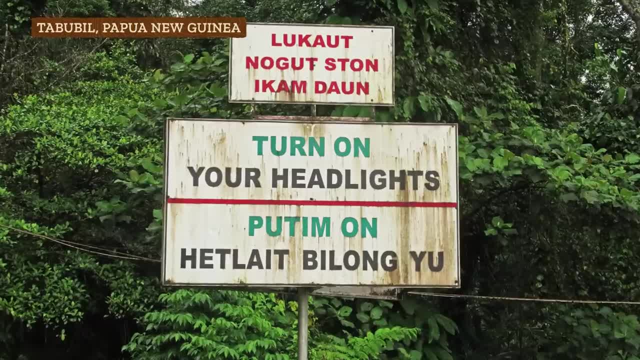 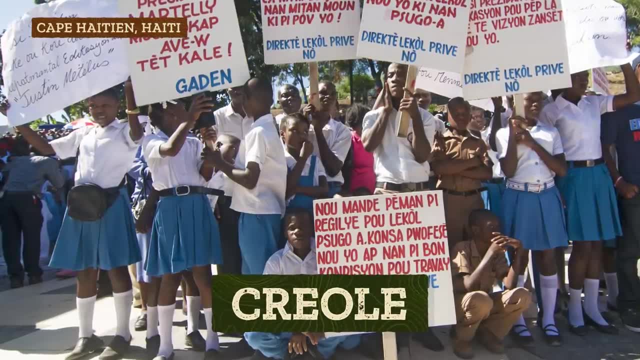 vocabulary combining two or more languages. Today, pidgin is spoken in places with a lot of language mixing, like Nigeria and Hawaii, And Creole languages, which are like leveled-up full-language versions, are used by people often in former colonies in places like Haiti and other islands around. 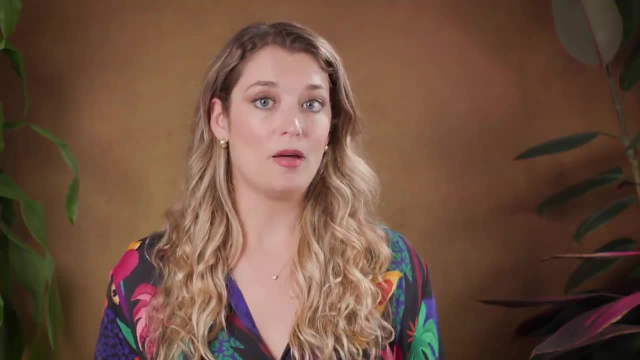 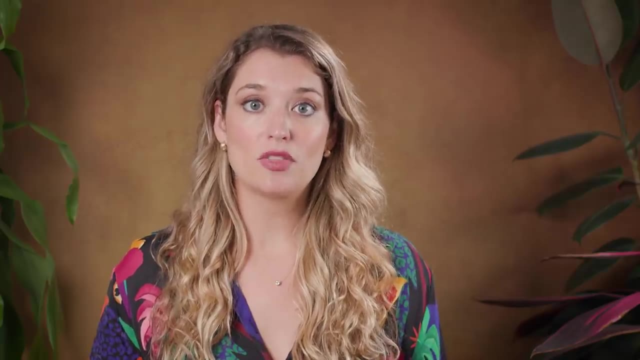 the Caribbean. Similarly, when people don't have a full language in common, they might rely on having a similar language origin, Like we have evidence that Africans who were enslaved and forced to migrate to North and South America used Bantu-based words they had in common to communicate. 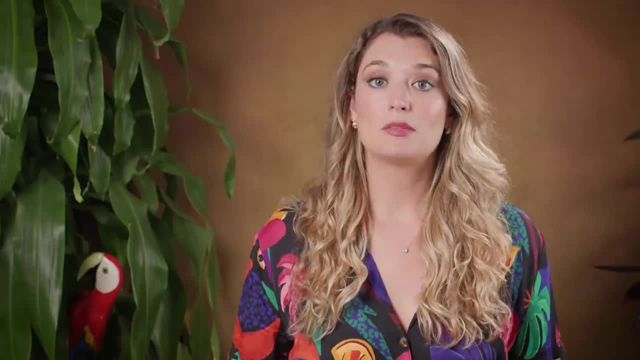 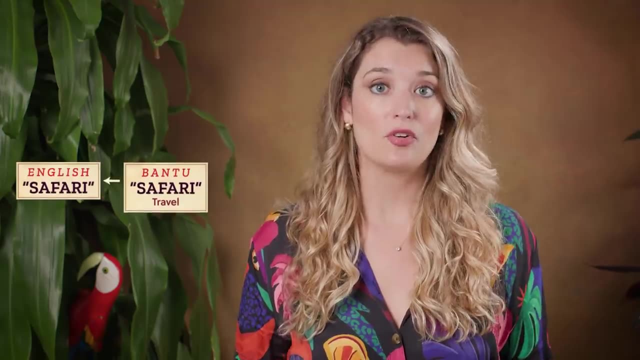 even if they mostly spoke different languages. And that theory seems plausible because of common words used in North America that seem to have Bantu roots, Like safari, which in the Bantu language, Swahili, means travel, but Bantu speakers may have gotten from Arabic. 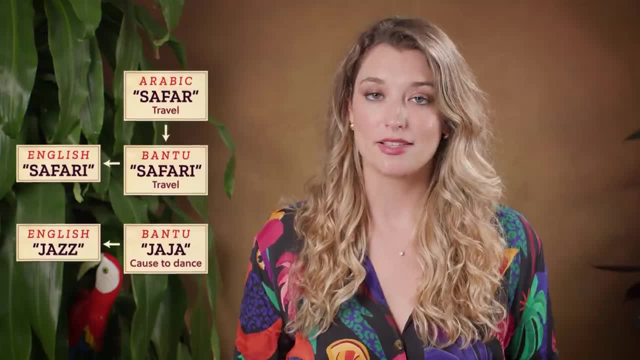 Jazz, which could be from the Bantu word jajah, meaning cause to dance, Or banjo, which is similar to a Bantu word, mbanza, for an instrument with strings that are plucked. But even a few words is enough to transport so much more As people move they're able to use. 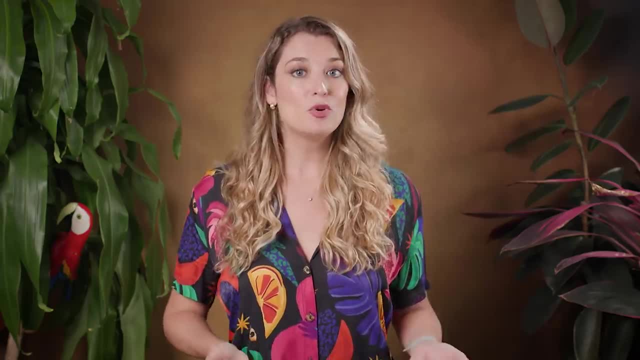 a few words that are similar to a Bantu word- mbanza for an instrument with strings that are plucked. But even a few words is enough to transport so much more. As people move they're able to use. As people move and language diffuses, they naturally carry all the other innovations a. 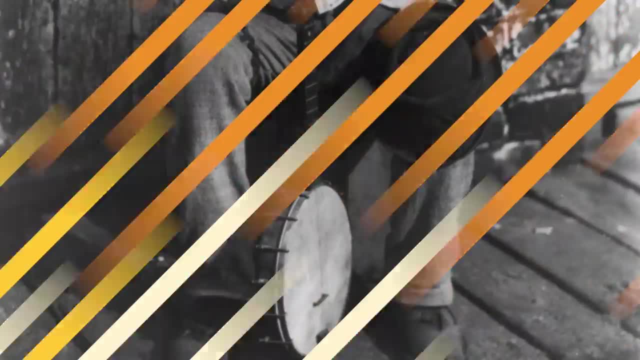 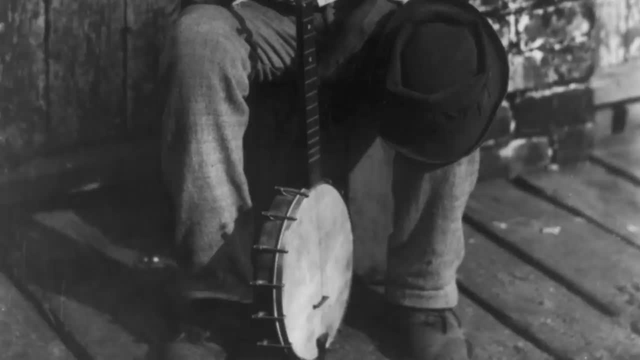 culture has especially stories, art and music. Instruments like the modern banjo have roots in the nations of Africa. As Africans were enslaved and forced to move, they brought that knowledge with them and found ways to make similar instruments and similar sounds to the ones they had in their 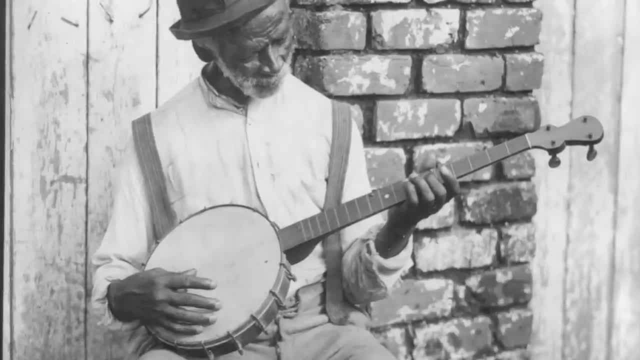 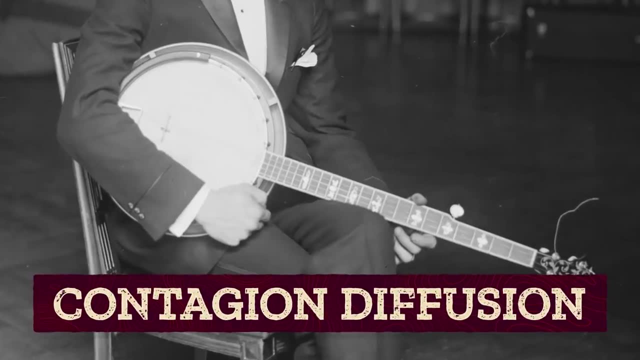 homelands. People across North and South America heard that music and slowly the music of the banjo transferred and spread to those outside of the African cultural groups. We call this contagion diffusion, which is when innovations spread just by exposing others to a new idea or object. 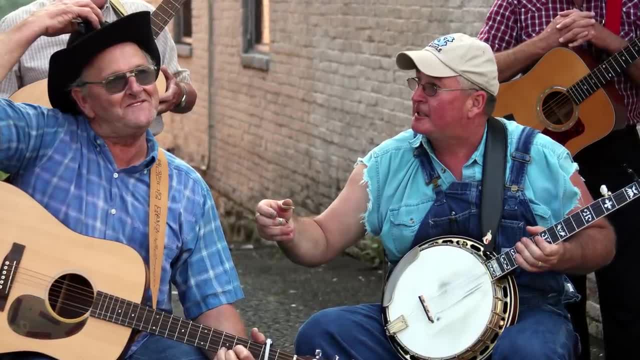 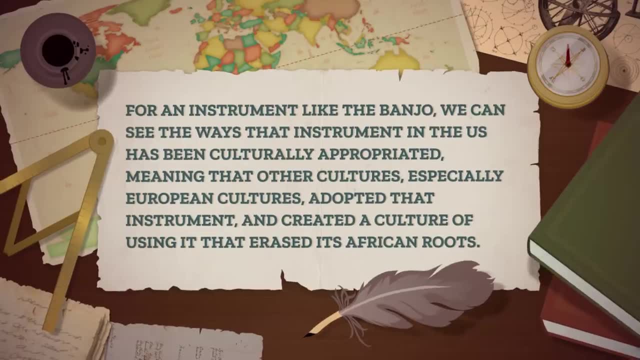 I actually just learned the banjo has ties to Africa this year, which was really interesting when we think about how it's so widely used today in types of music widely associated with white people like traditional bluegrass. For an instrument like the banjo, 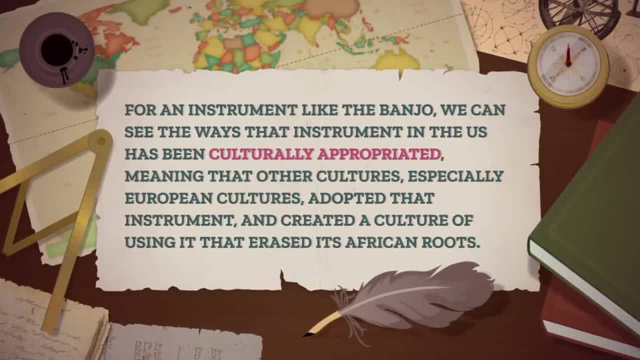 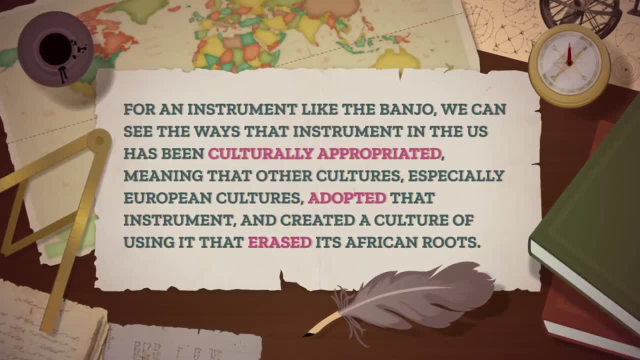 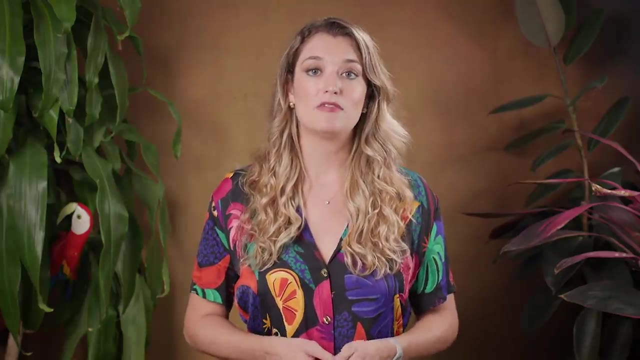 we can see the ways that instrument in the US has been culturally appropriated, meaning that other cultures, especially European cultures, adopted that instrument and created a culture of using it that erased its African roots. Cultural change is inevitable. As we learn and grow, each generation is often taught slightly different cultural traits because of 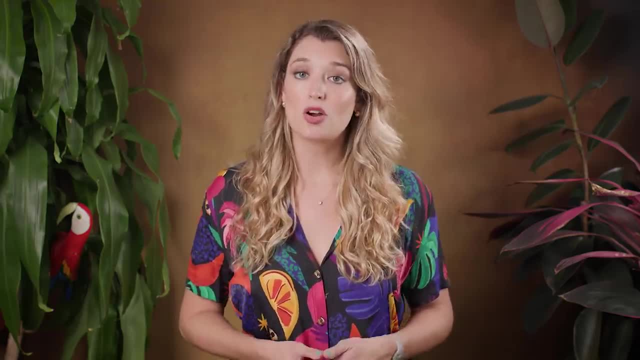 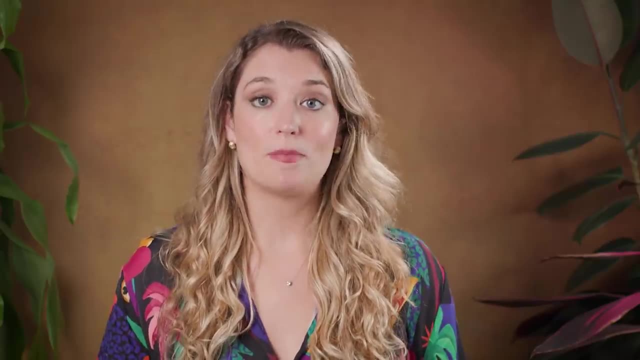 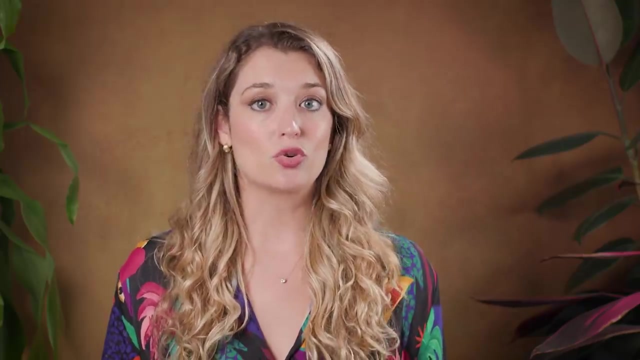 mixing and diffusion. and as people move around this globe, so do our cultural traits. Every interaction creates a new space for growth, innovation and change. But restoring cultural connections to the past, like dormant languages, and historical connections to current cultural traits, are important too. Those efforts restore cultural ownership. 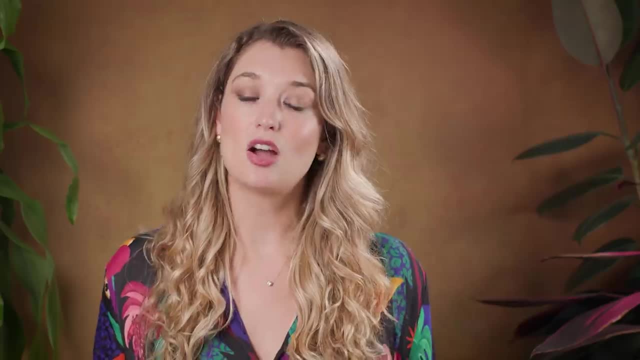 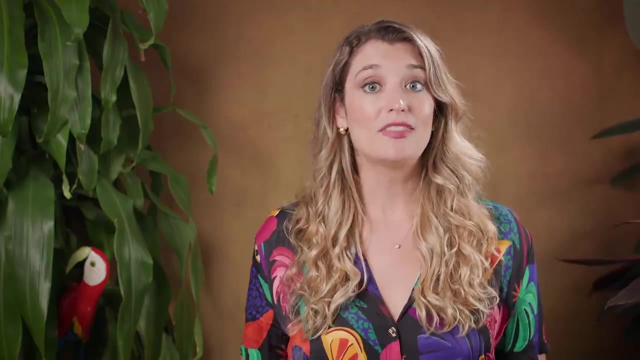 and help those inside and outside of those communities to recognize the contributions and humanity of our world's cultures. Understanding the movement and diffusion of language helps us understand other cultures, get their jokes, see the world as someone else and understand how so many other cultural traits move. And next time, 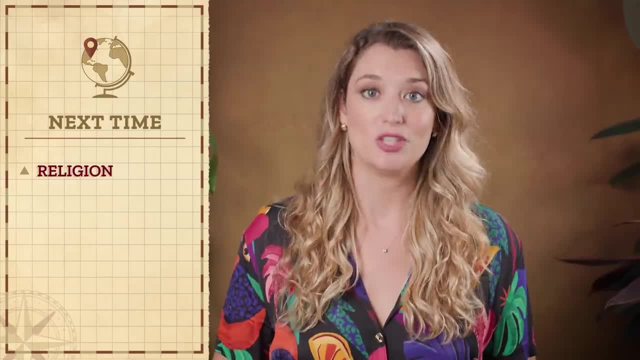 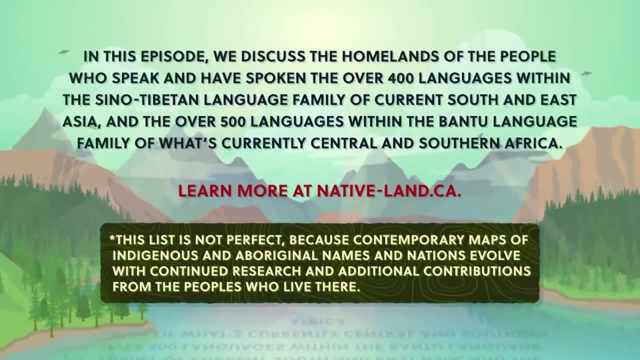 we'll explore the movements of one other major cultural trait: religion. Many maps and borders represent modern geopolitical divisions that have often been decided without the consultation, permission or recognition of the land's original inhabitants. Many geographical place names also don't reflect the indigenous or 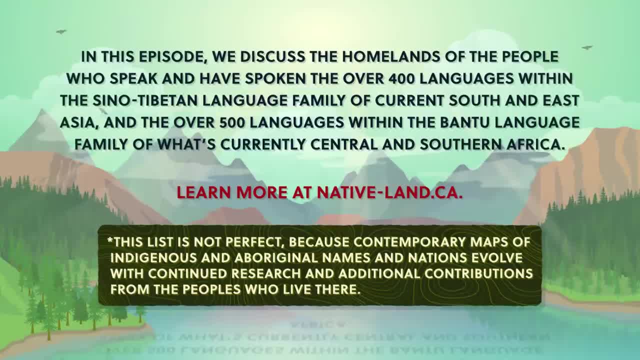 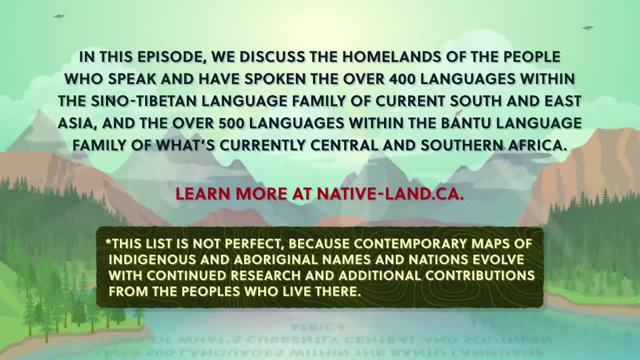 aboriginal people's languages. So we at Crash Course want to acknowledge these people's traditional and ongoing relationship with that land and all the physical and human geographical elements of it. We encourage you to learn about the history of the place you call home through resources like